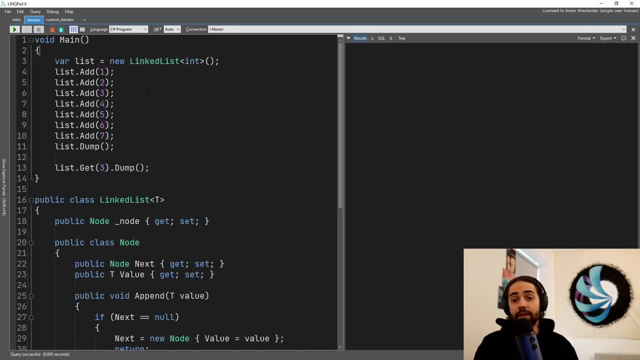 on. this link is in the description, so let's dive in. if you're going to enjoy the video, don't forget to like, subscribe, and if you have any questions, make sure to leave them in the comment section. here you can see me using the linked list. we're adding a bunch of items. we're then dumping the. 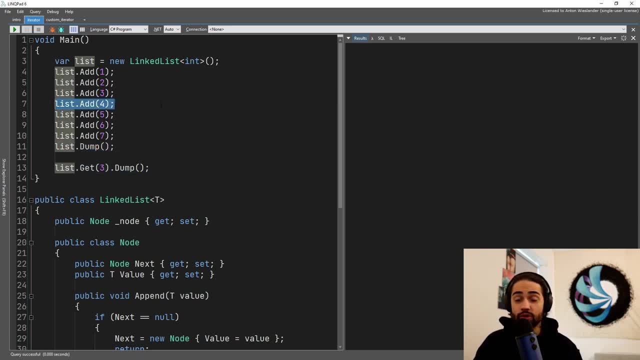 list and then we can also get a third item, which is going to be this number four. we give it a run, then we're going to go over the iterator pattern and we're going to go over the iterator pattern, and we're going to go over the iterator pattern and we're going to go over the iterator pattern. 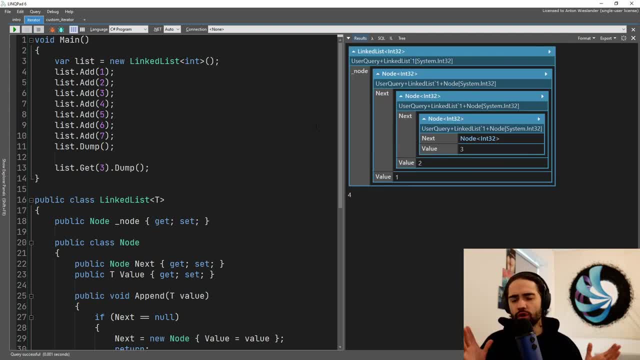 this is what it looks like, so we have a illusion of a list. so things are in line. you can see there's kind of a little bit of a nested structure is, but that's just how it's displayed in the ui. we'll go over the implementation in a minute, but essentially we have a linked list. 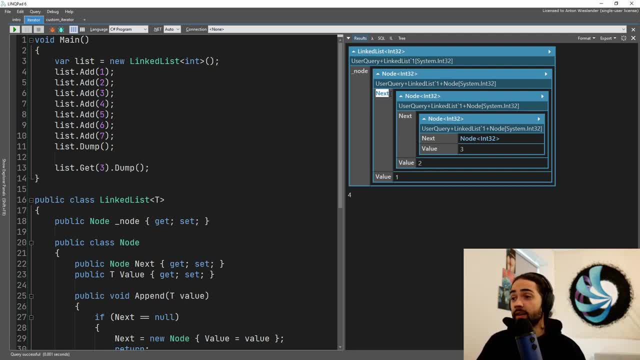 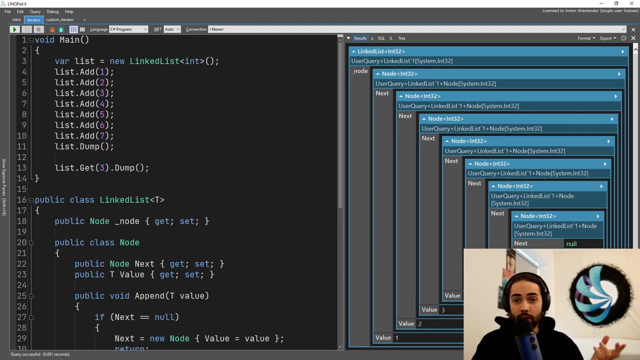 that has the first node, the root, the start of the list, which contains a pointer to the next node, but itself it contains a value. so the next node contains a value and points to the next node, and so on and so forth. they keep pointing to the next and next node until we have the number seven. and if you're wondering, why wouldn't you? 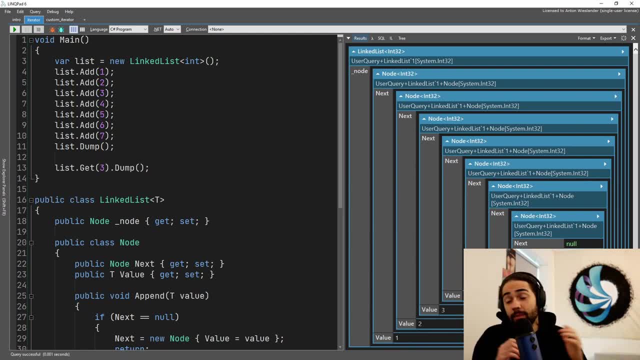 just use arrays instead of a linked list. if you've ever started programming and you're like, oh man, why can i not change the size of my array at runtime, well, this is the reason, right. this is infinitely scalable, as long as you've got the memory and the things. but you can just keep adding, removing and. 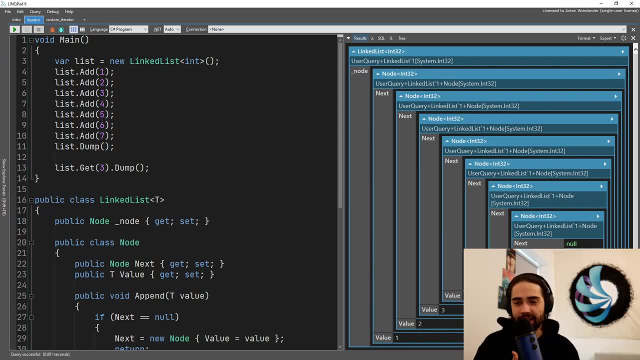 the size of the list is dynamic. if the array and the linked list are both hidden behind the innumerable or iterator is the same. you can just keep adding, removing, and the size of the list is interface. it doesn't matter what you're iterating over, the performance maybe slightly different. 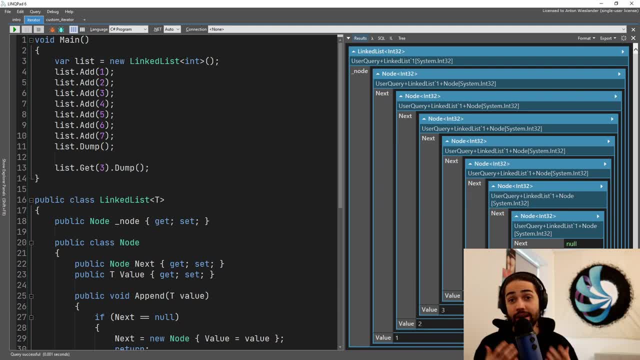 the way that lists work in c sharp is they use arrays internally and if you do exceed the bounds it's just going to go ahead, do an array copy and reassign it and use a bigger size, right? so there is a slight overhead there for the convenience of the indexing that it allows you to to use. 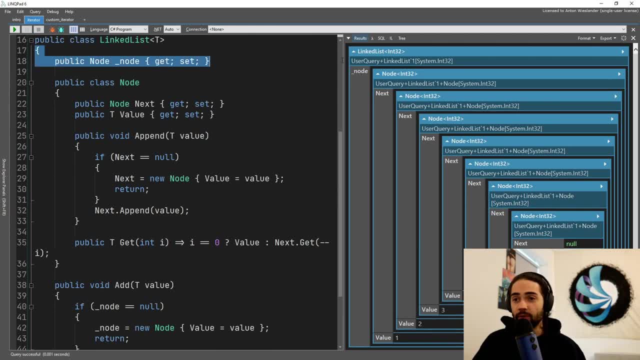 anyway, let's go through the implementation a little bit. so we have the nodes, those are the things that keep. this is the start, and the node itself is the one that keeps pointing to the next value, and so sorry, that points to the next node and contains a value itself. we have the append function to append a value as being the. 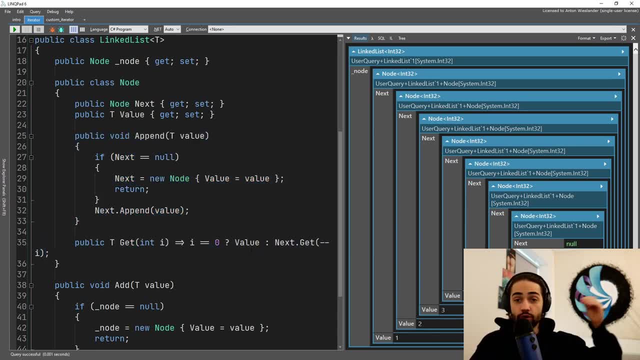 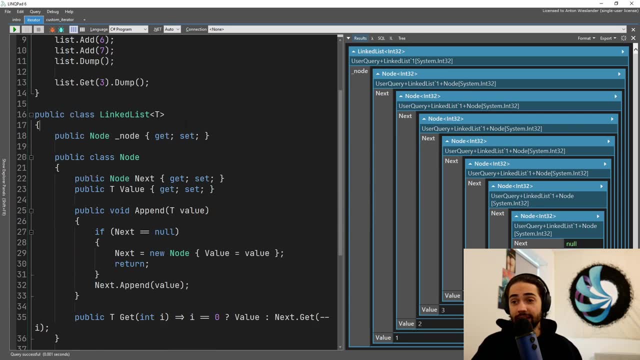 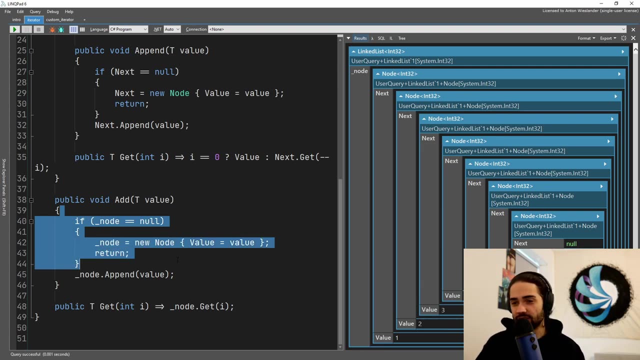 next node and the get function in order to grab a value at a certain index, and that is what we're doing here. the initial add and get functions on the linked list itself are just proxies into the actual node and the initialization initialization process. essentially, this is the base structure, just going over it here before we jump in and try to. 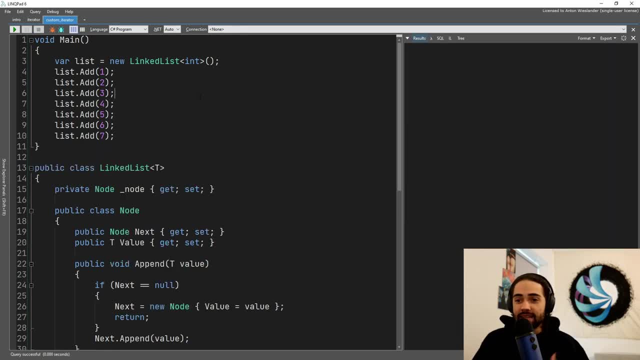 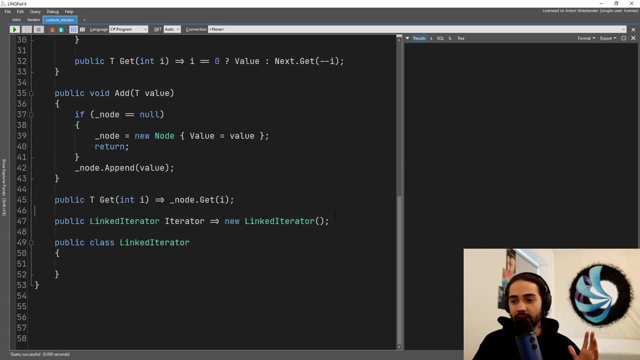 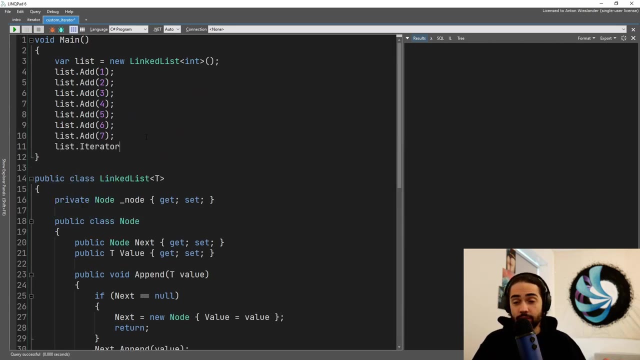 bolt on an iterator into here. same setup. i have the same linked list. at the bottom i have added my linked iterator and all i'm gonna do is i'm gonna call list dot iterator and that is going to give me a new object that is going to contain the state for the iteration over the list or an. 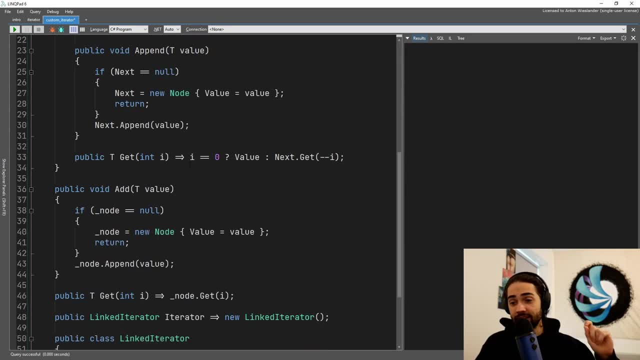 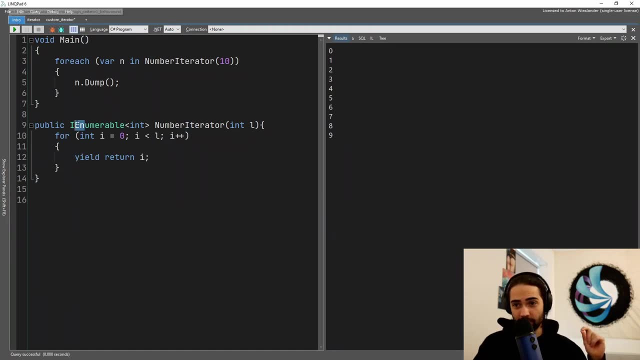 aggregate. the main purpose of the list is to give me a new object that is going to contain the state for the iteration over the list or an aggregate. the main point that i want you to take away here is that this linked iterator is a concrete implementation. real iterators, for example, like innumerable. this abstraction is used over multiple types of 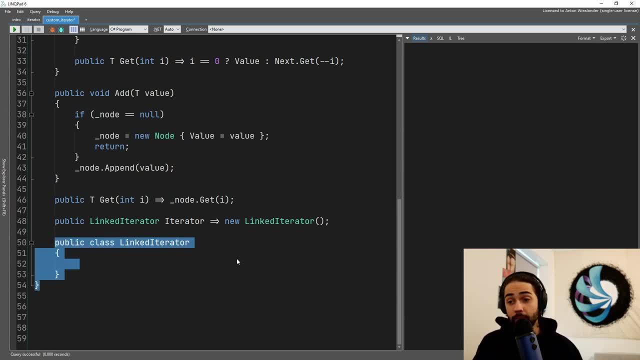 collections. okay, usually if you are going to implement an iterator, you want to hide it behind some kind of interface, so those specific collections have to implement the logic for that specific abstraction to work. anyway, here we're going to be working concretions. just understand that main point. you do want an interface, some kind of abstraction, so those concrete implementations. 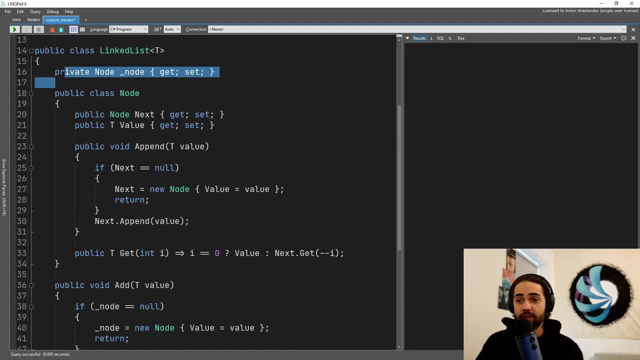 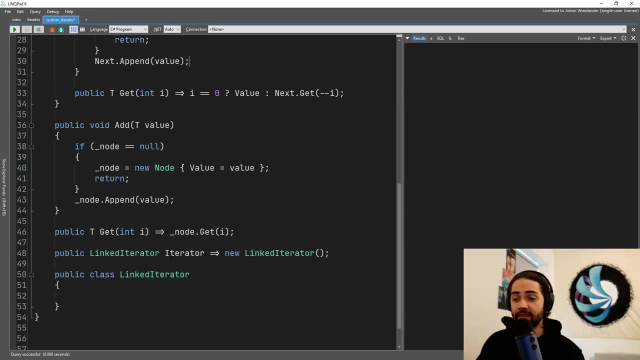 work against that contract. our linked iterator will need to be aware of the nodes, the actual items that contain the values, and that's what i'm going to start with. i'm just going to go ahead and pass in the node into my linked iterator. i'm going to create a constructor. first parameter should be: 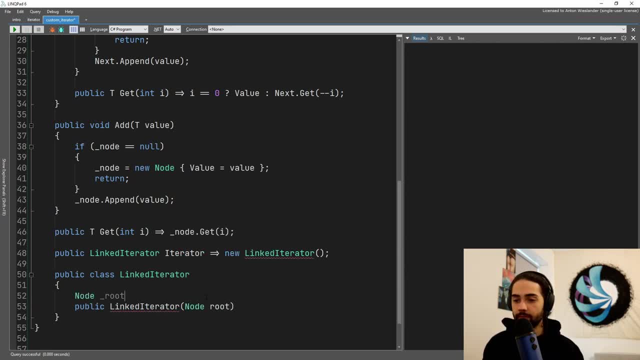 the root, the beginning. let's create a private field for root and now we can just assign root to root on the iterator. we can pass the very first node within the linked list and that's pretty much it. our iterator is now seeded with the collection that it should traverse. there are a couple of 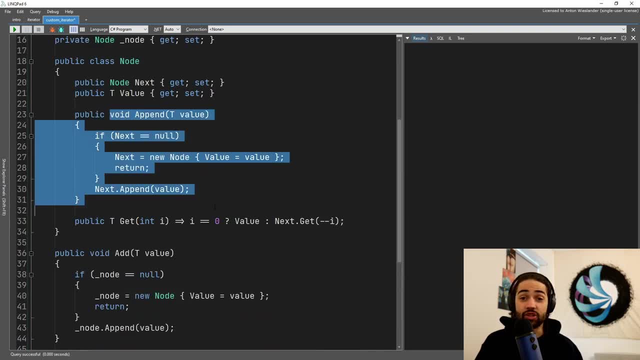 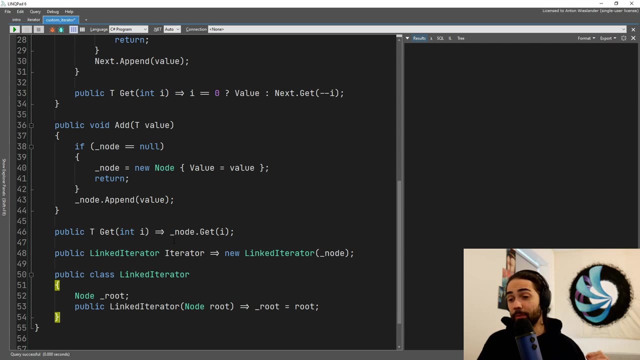 concerns here, like: what if the collection changes? we're no longer iterating over the same snapshot, and that is something to keep in mind if you're implementing the iterator, although that is not so much a concern for the iterator, to be fair, in my opinion, it is the developer that should be. 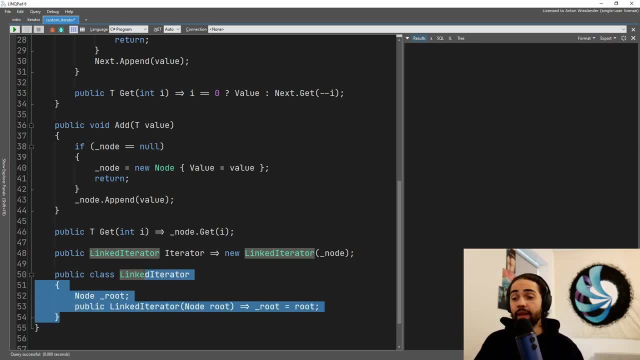 careful with how he manages state. let's continue here. we have the iterator that contains all the state that we should go over. let's traverse that state. let's say that whenever we try to get an item from the iterator, we are always going to get the items in their succession. so they are in some. 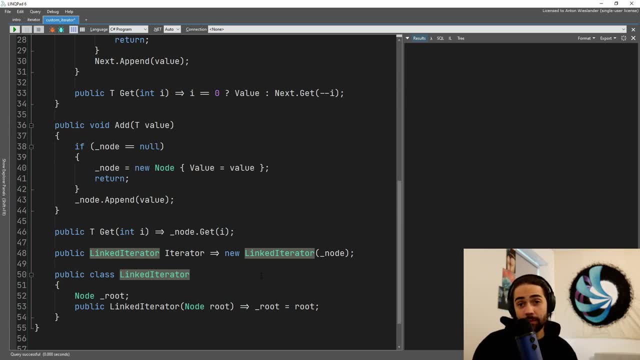 kind of order in the list. every time you say, give me an item, it is going to automatically iterate over it like a for loop. that is essentially the behavior that we want to do in the list. let's see how we can do this because we have this node structure. it is going to look a little bit. 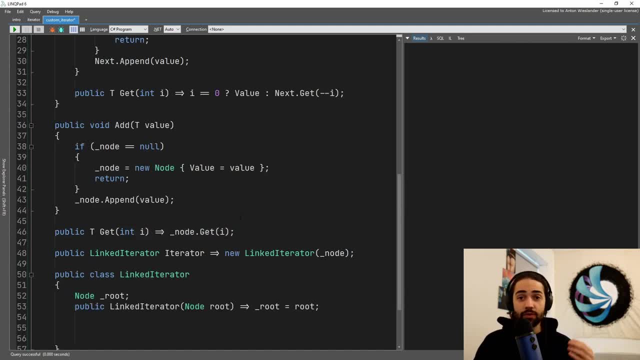 different and instead of keeping the index and having this inefficient lookup from the beginning to the end, i'm just going to store the node on which we have currently stopped. this will require me to hold the state for the node that we currently are trying to grab the value from from the beginning. 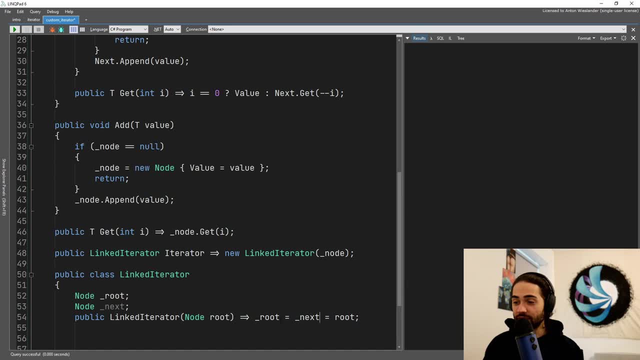 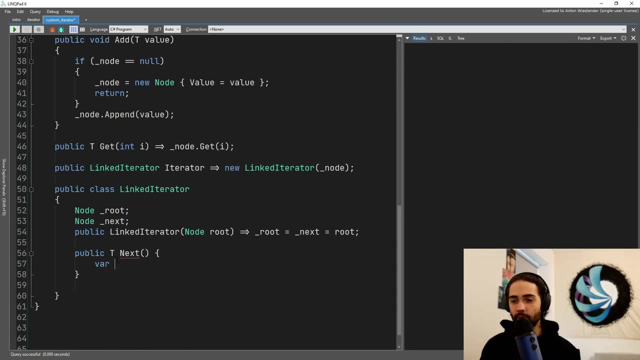 we're gonna start from the root. so in our constructor we can assign the root to the next node and then have the next value where we will grab the value from the next node value. so initially we're going to grab it from the root. at the end we will return the value. we will then 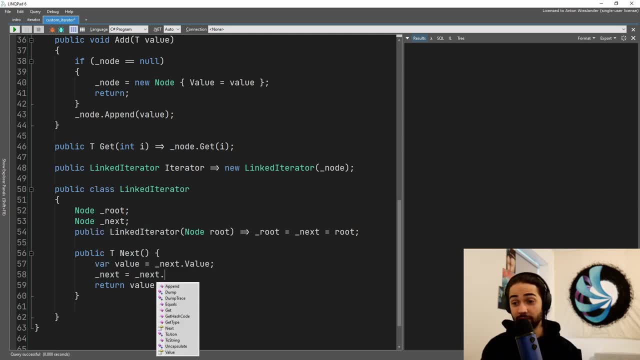 go ahead and assign the next node to be the next of the next right. so that did sound a little bit weird. so maybe it's a little bit clearer if we use current instead. if we then try to go and perform a reset, this would look something like setting the current to the root. so we just take whatever item we're. 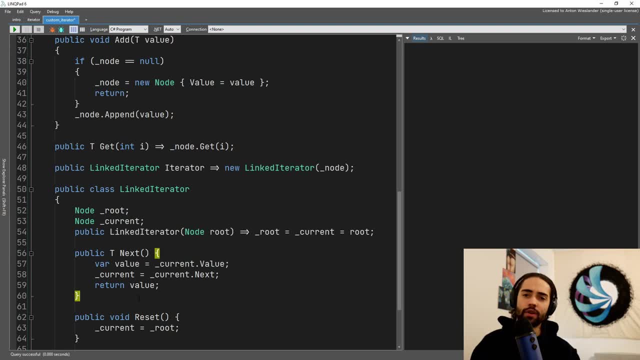 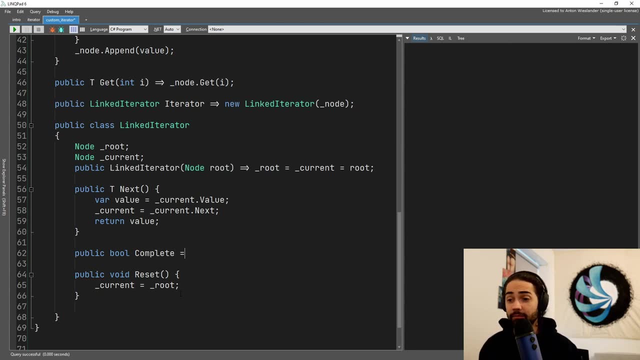 currently pointing to and just say: go to the beginning dude. and, of course, another function or property that you can implement is a boolean of complete. are we finished iterating, are we not? i would say the only time that we can know is if the current one is set to null. the very last item. 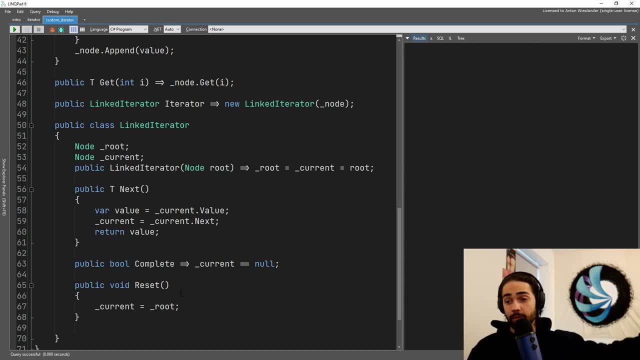 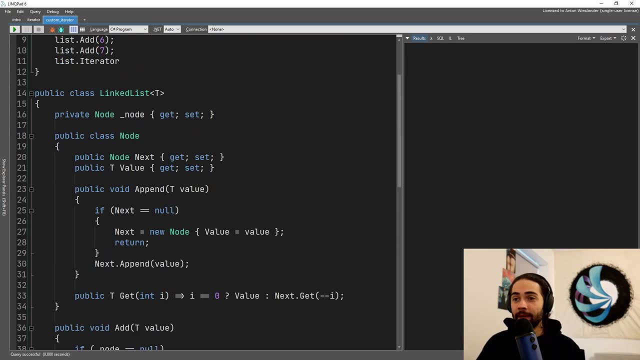 in the linked list is going to be pointing to nothing once we go ahead and assign that nothing to current. that's what we're going to do, and then we're going to set the current to null, and that's what we're going to end up with with. we're going to end up with null. how will this look?